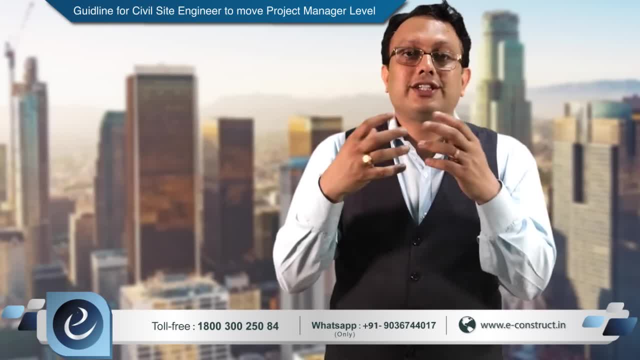 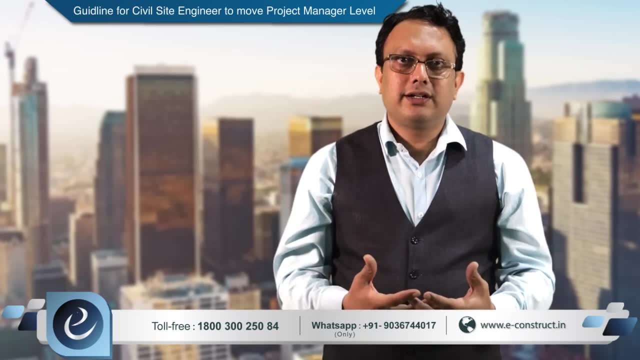 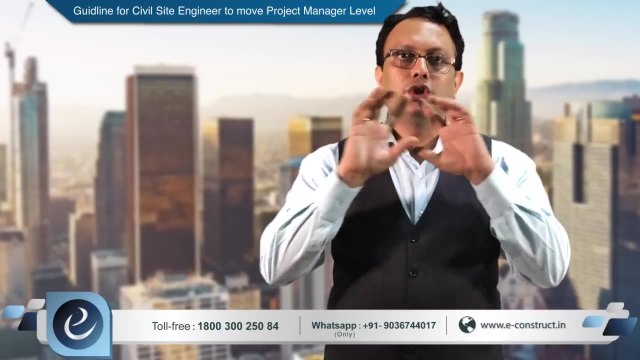 that. what are the technical skillsets and behavioral skillsets And what is skill? Skill is something like: what are you expert at? That's a skill right To become an expert or to become a skilled person. you really first and foremost thing that you need is knowledge. 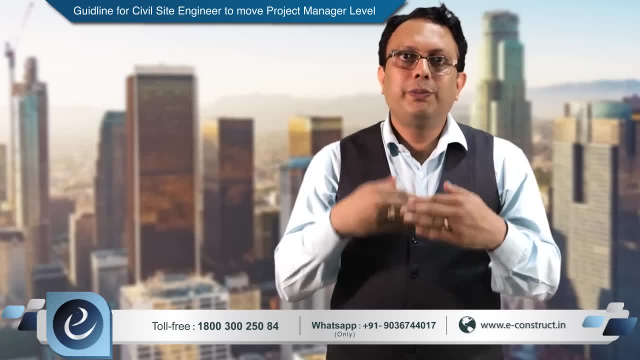 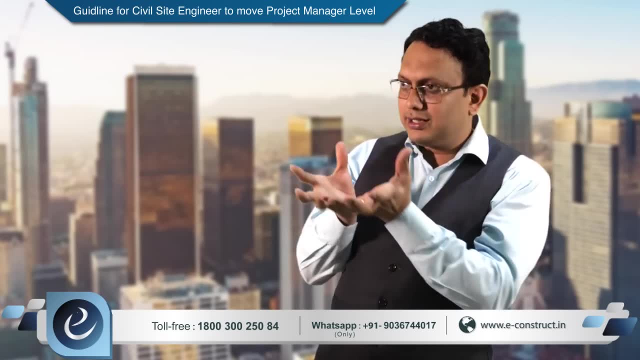 First of all, you should know that what is the knowledge that requires first to become an expert in that. Let's say a camera, For example, or let's say anything which is related. for that sake, You first know what does the camera mean, What's the mobile mean? What is Android mean Initially, if you remember? 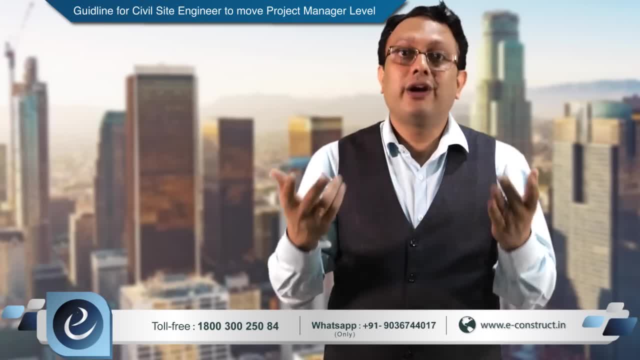 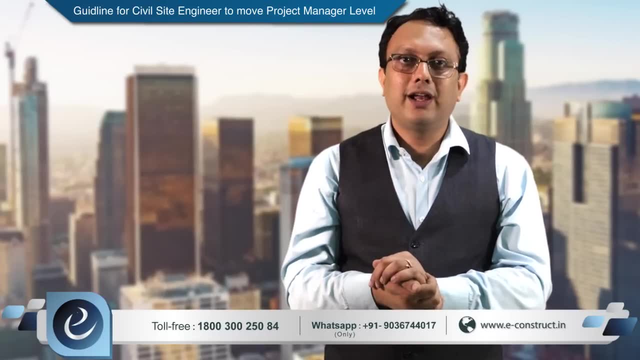 before the mobile phone has born, you might be knowing what is Android. Nobody was knowing. Now, everybody actually, even the three years, four years kids actually are playing with the Android mobile right. But if you see that, oh, very old age people like your grandmother- 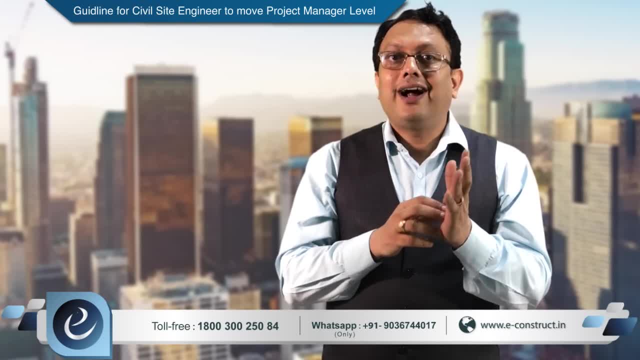 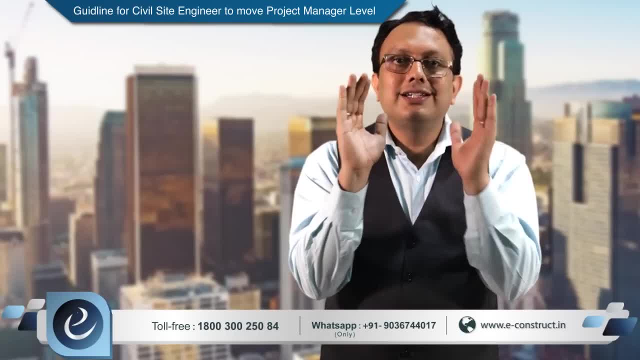 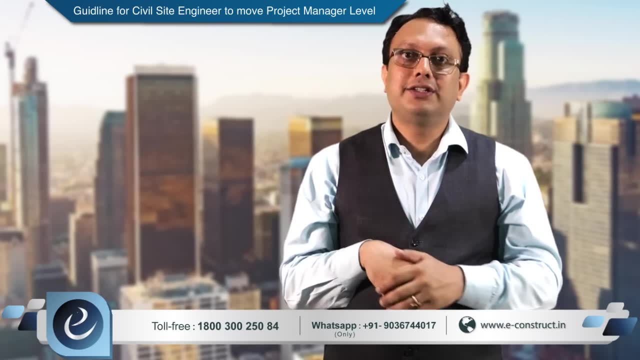 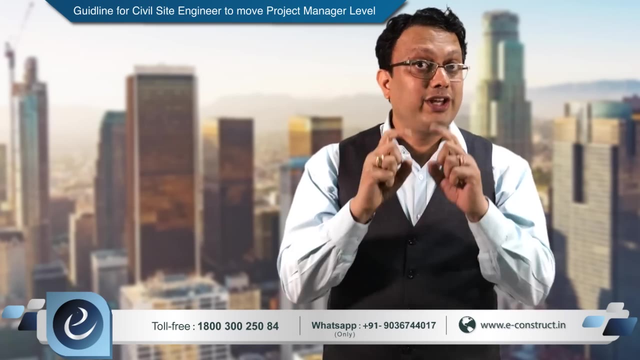 quota or their doors of acquiring the knowledge has completely got closed, right. So one thing: you please make sure: make a statement in your life that you will never, ever close the doors of acquiring the knowledge. all right, That's a very good quality for a project. 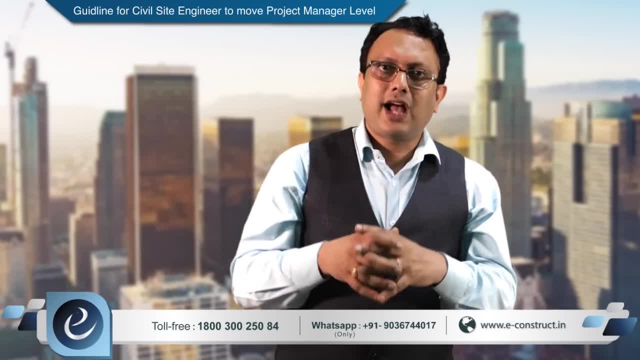 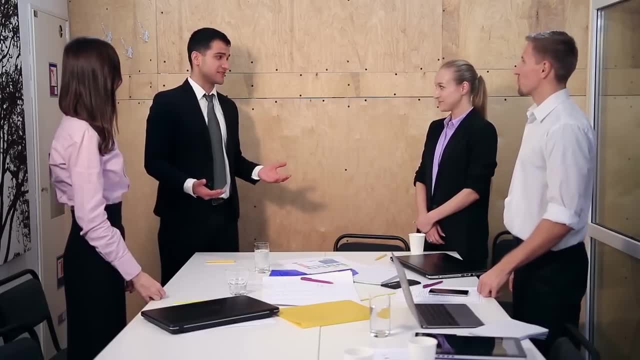 manager, Few qualities or few skill sets- How to categorically define it? Now let me talk to you about the, the behavioral skill sets. behavioral skill sets is: first, is you should have a communication skill. now, where are you getting stuck? are you getting stuck with? 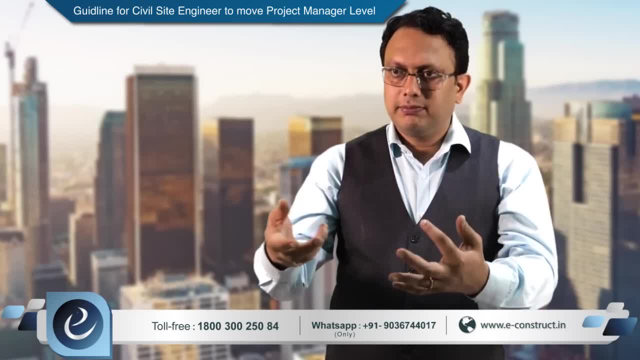 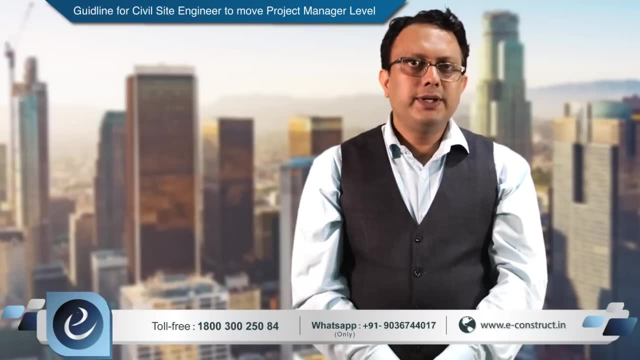 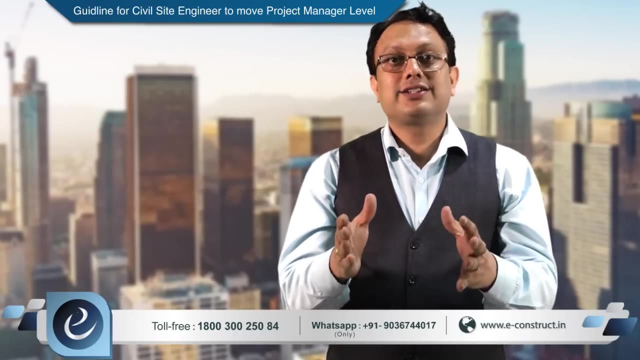 the local language? are you getting stuck with the national language? are you getting stuck with the international language? somebody will say that I am a Gujarati. I will speak only in Gujarati and I'm a Marathi. I'm going to speak only in Marathi. that won't work language. please understand. I'm not favoring any. 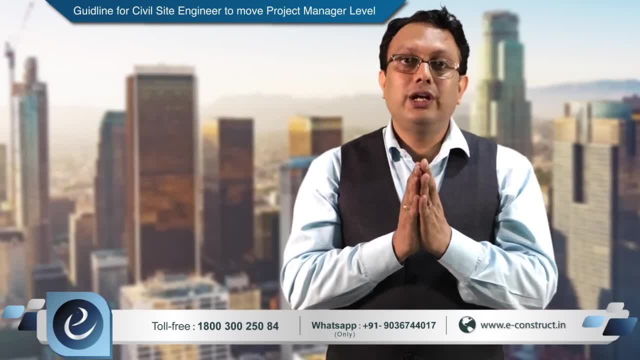 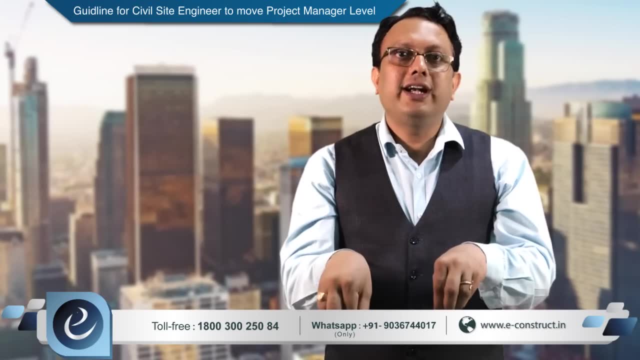 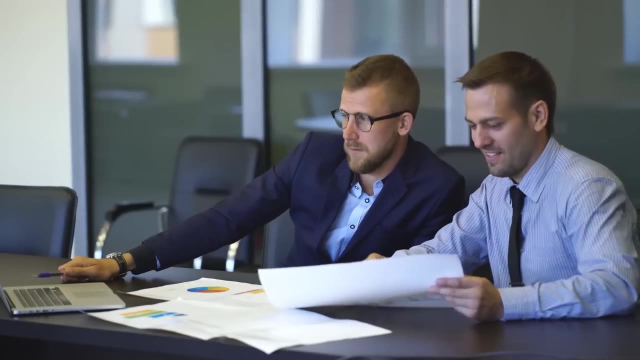 language or I'm not favoring English language. I'm just trying to tell you it is the proper communication between the two people, without having any deficit of the content or the knowledge. all right, one person wanted to tell something to other person. it has to be communicated along with the feelings, along with the 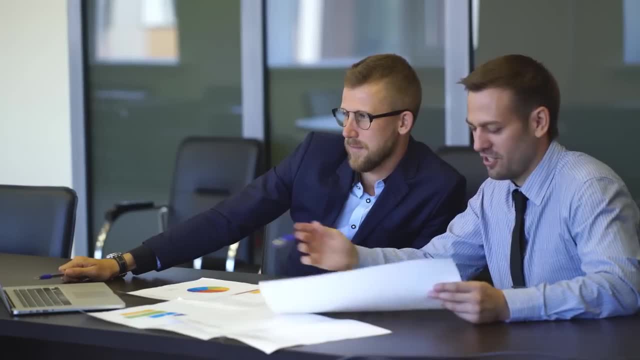 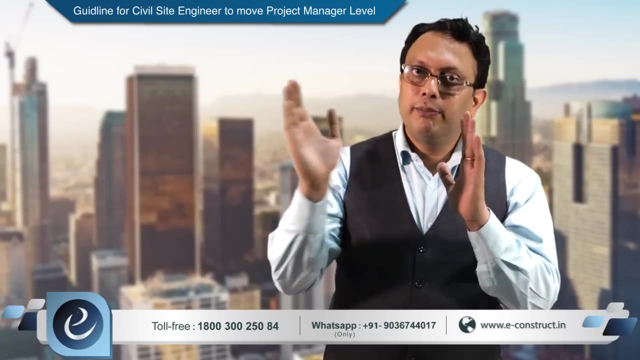 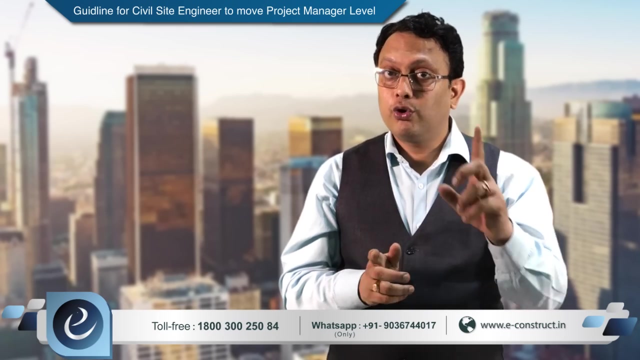 technical details, every damn thing. that's the knowledge you tell him like without speaking. also, it's okay, but a proper way of communication is the proper way of communication. which kind of language? so coordination, communication skills, you really need to have it. if you don't have, get it right away, right now. how to get it? the 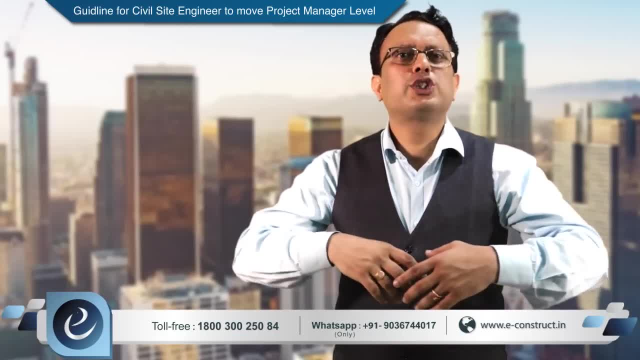 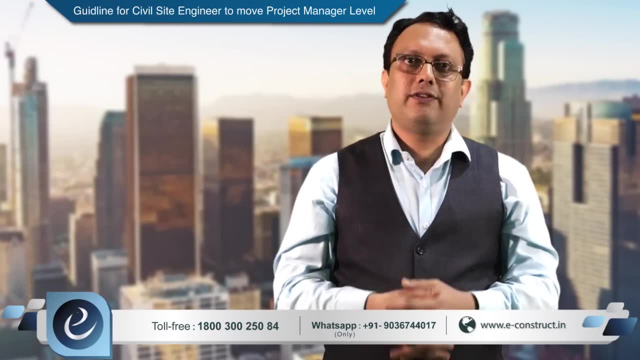 communication is. it's very difficult. there are so many people they cannot speak. if you really want to speak something, actually try to sit in front of the mirror. speak something about yourself. speak something about the subject that you are loving for. speak something about of the person to whom. 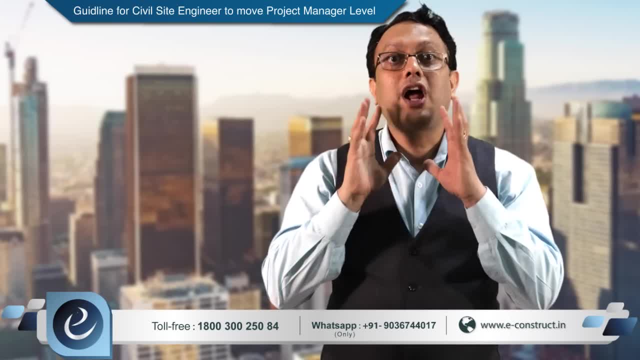 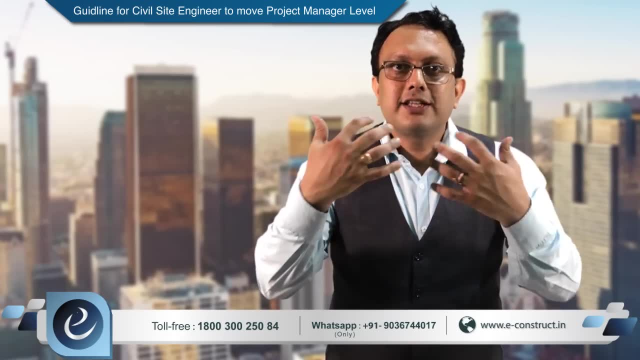 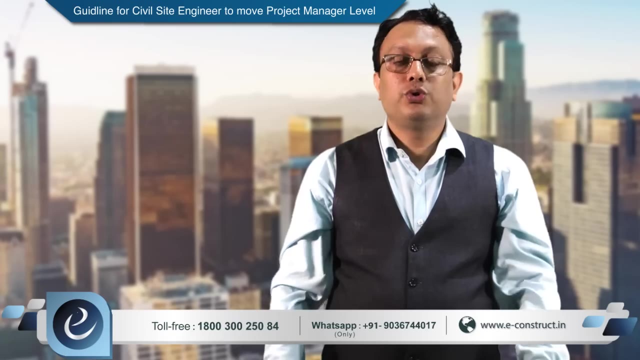 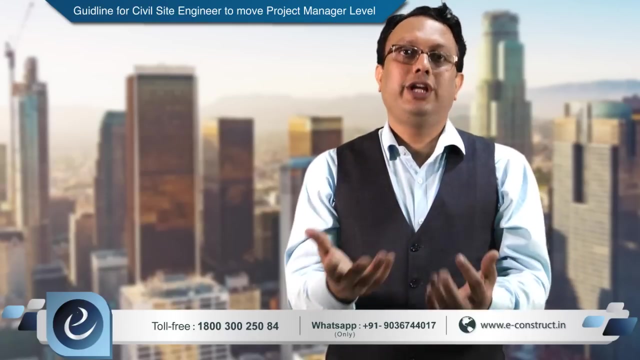 you are loving for something or something, actually try speaking outwardness. outwardness, it's very important. there are some people which are introvert. they speak internally. there are some people they speak outward. so you required to be a little bit more outward spoken person. it helps you communicate right. so communication skills: there are few areas. 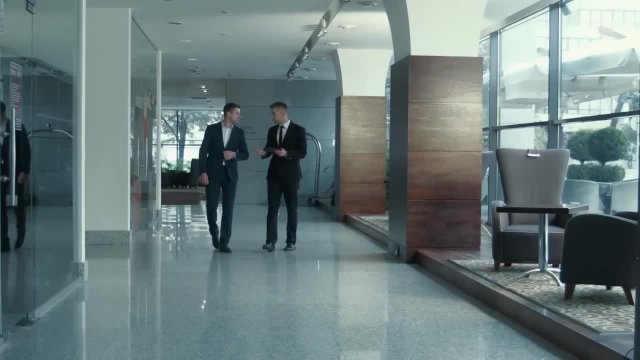 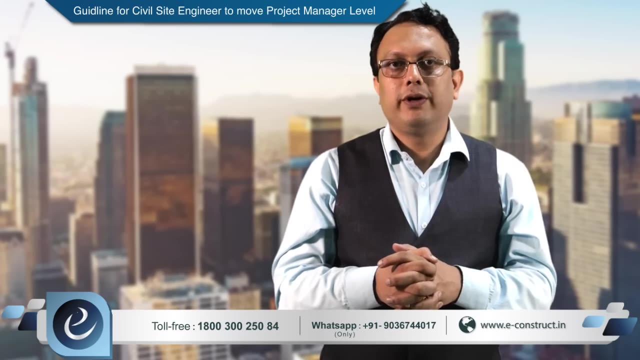 actually I just want to tell you, communication doesn't happen only with the speech. communication doesn't happen only with the speech, it happens with the body language, right? so those areas also you need to work a little bit more. another area: the the cutting the behavioral skills, I'll tell. 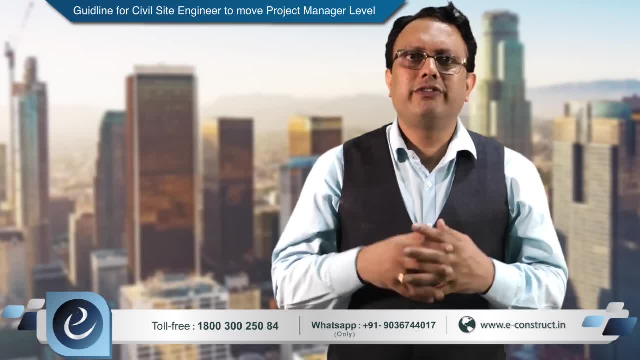 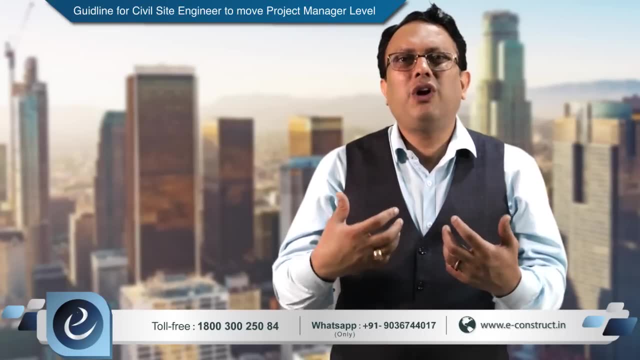 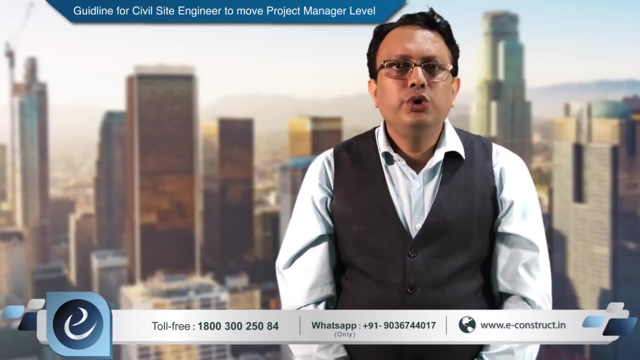 you motivation. you really need a self motivation. there are so many, so many moments will come in your life that you will not feel any motivated. you will feel very disgusting also sometimes. so what do you do you? do you do something which inspires you from the zaoling all these things in the Bar黴. 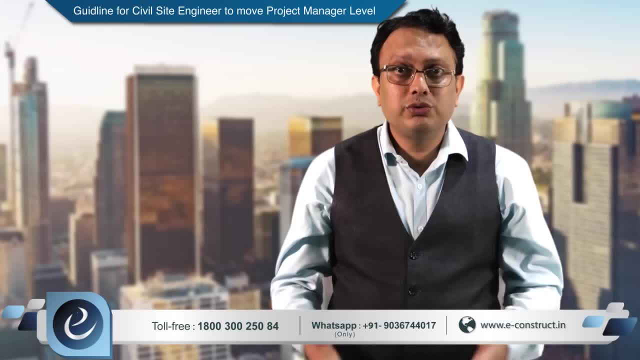 also givesлись this goal and creativity what you need in your life, the path for you. what's the path to reach a? you will also have to. within all right, you do meditate if you really want to do that. you pray, you go to some church, you go to some temple, go some places where you will feel joyful. 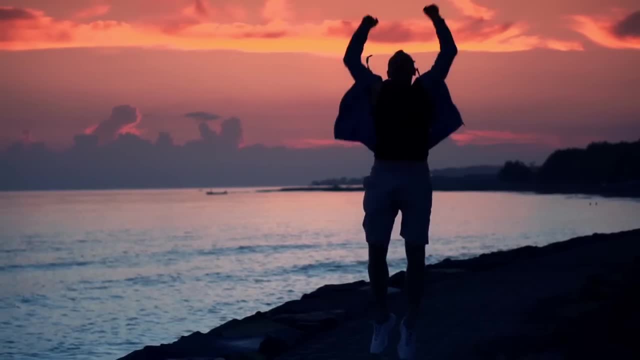 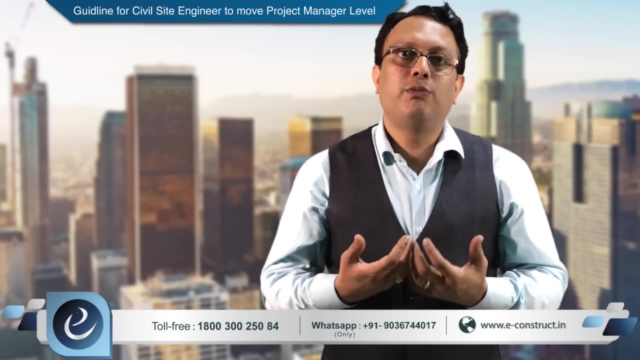 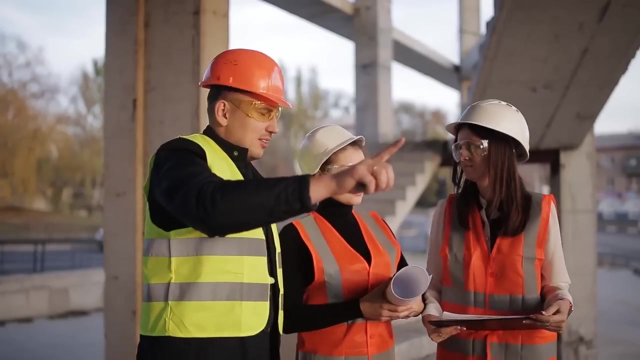 where you will feel happy about, where you'll feel very enthusiastic about. so this is the key area where you really need to be self motivated. if you are not motivated, how you can motivate other people, how you can motivate your colleagues, how you can you motivate your- you know- labor staff, other staff or 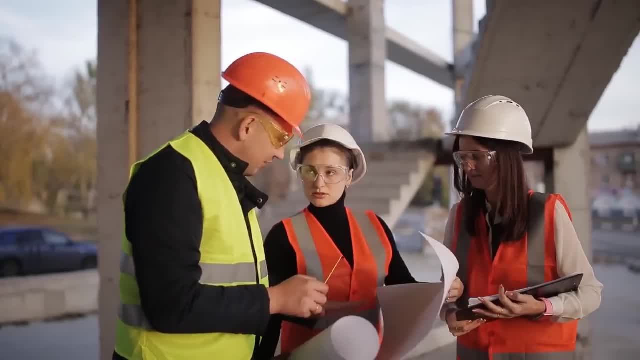 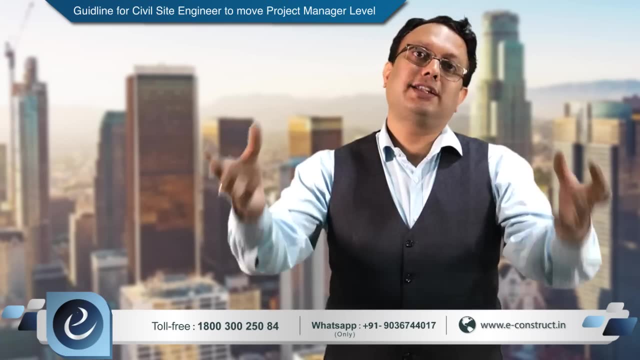 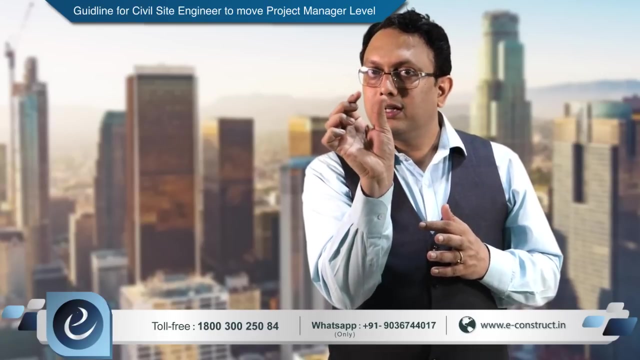 engineers, architects project. you know the site: engineers- so many other people you can't motivate. so self motivation will inspire you to motivate other people. all right, that will drive you. that will reduce the span of the work that is to be carried out during the certain activities. believe me, it helps. 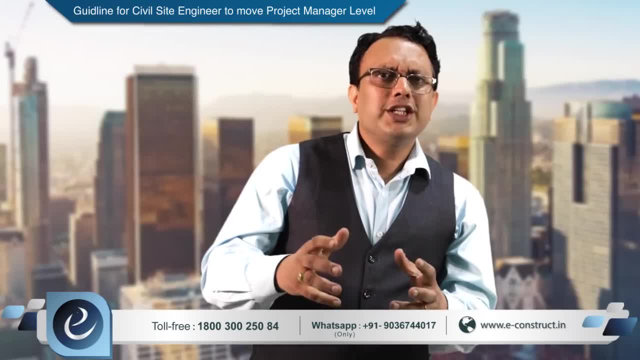 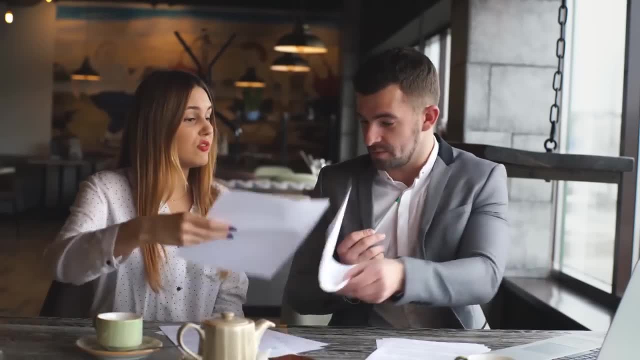 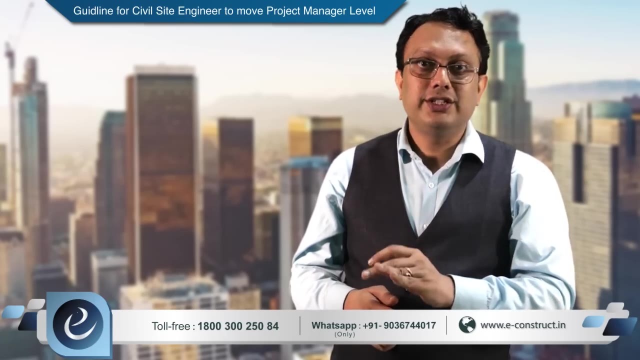 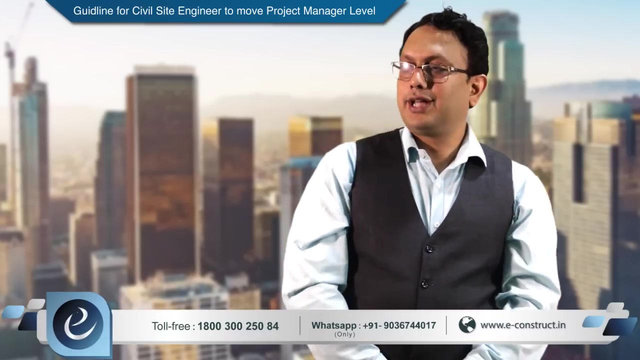 certain other activities are like problem-solving. you know that there are certain issues are happening here. you should look at, not the problem, at the solution. you are problem-solving person, not the problem creator. now, this is very important for so many civil engineers. they become a problem creator, sir, this is not there, sir, this is a problem, so that is a. 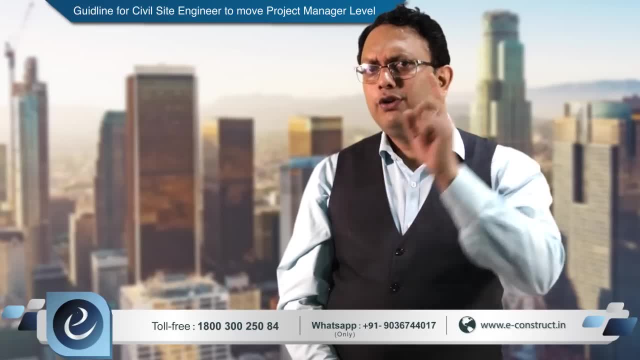 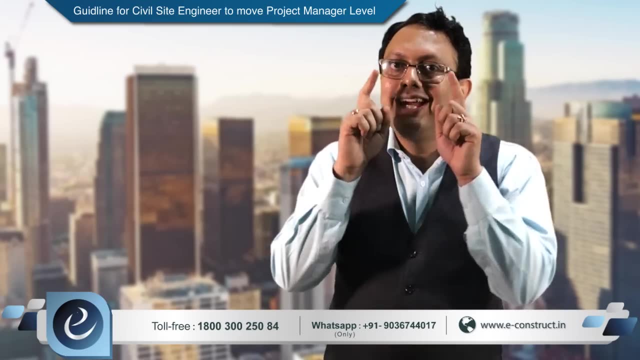 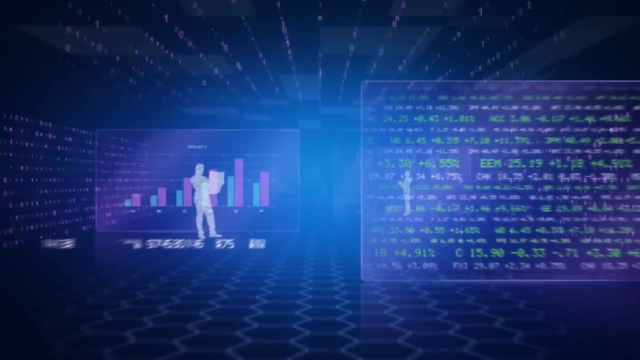 problem. no, if you are a site engineer, if you are a civil engineer, you always and always try to find out the solution to the. this is the key principle for you will take you to the places: from problem to the solution, problem to the solution, and number of problems are there on the side. 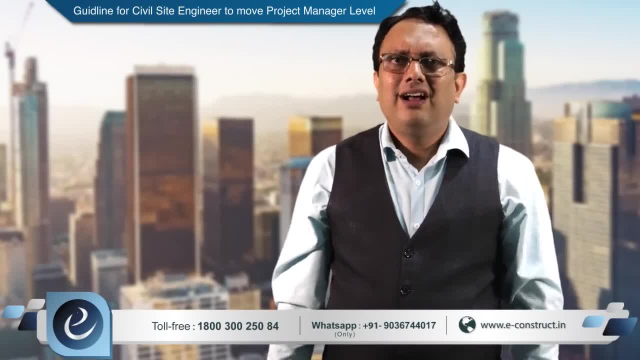 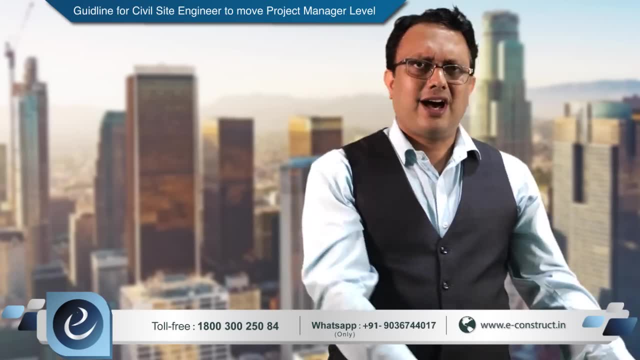 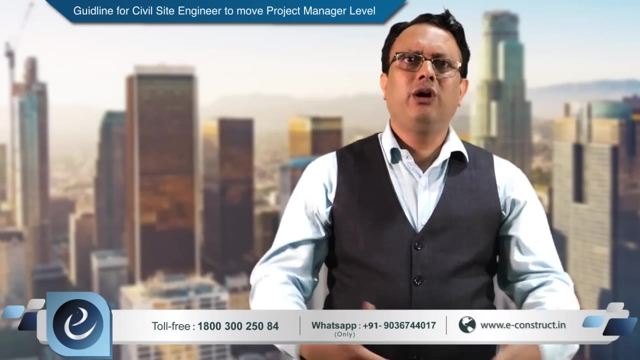 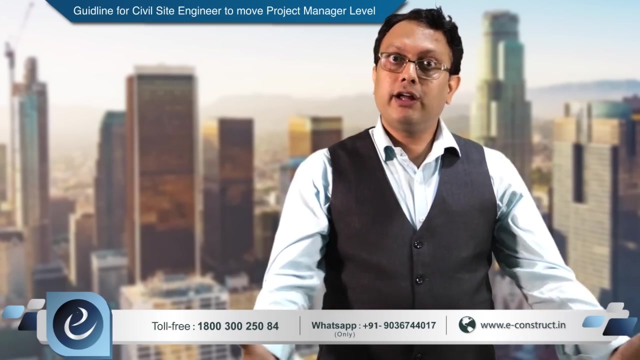 people are getting frustrated. when my site will get finished. what this bloody engineers- architects, mechanical, electrical, plumbing, IT- so many consultants- what the heck is going on when my project will get over? why? because I have invested on land, crores of rupees. I've invested on construction. 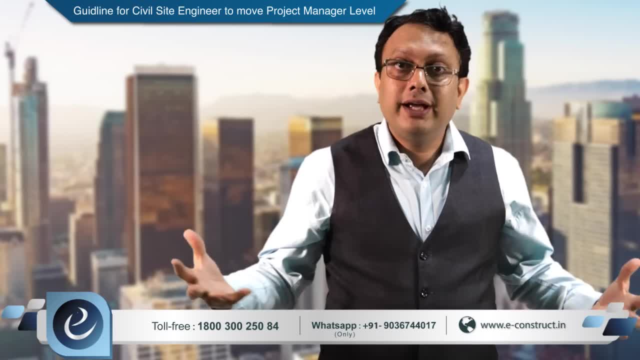 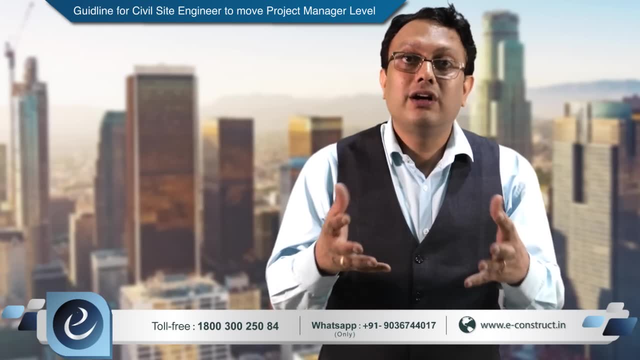 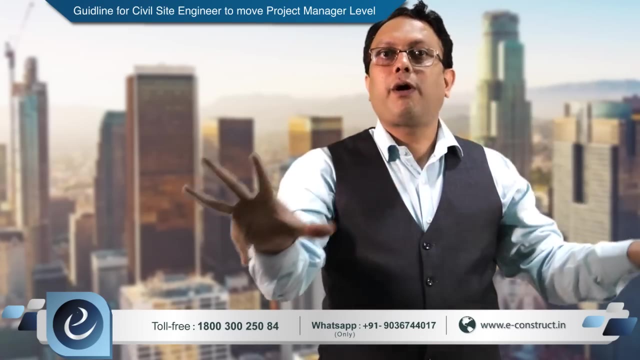 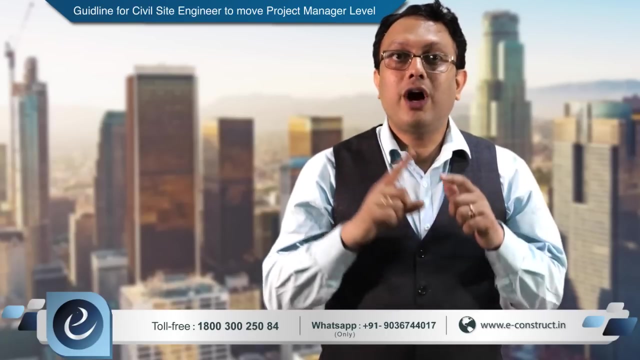 millions of rupees. what am I getting? nothing. these people are fighting when I will complete my project. that's very important. all right, so you become a solution orientation person. don't try to enlarge or magnify the problems. try to kill it, try to curb it. try to resolve it and make a proper solution. you are the. 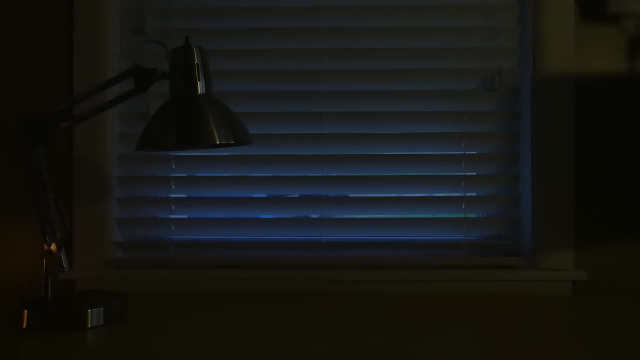 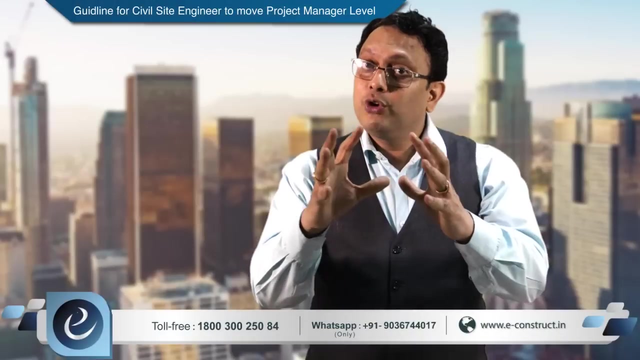 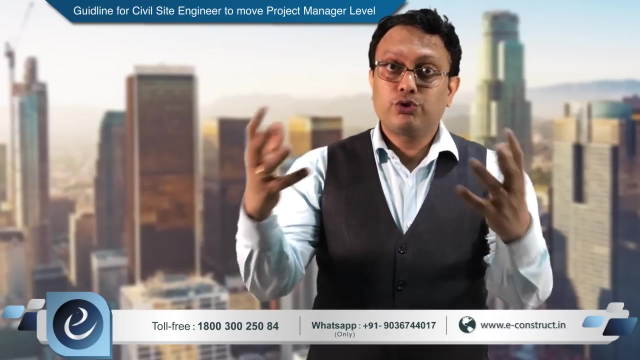 solution, orientation person, and you know that better. next quality is team building. what is team building now? team building is a very, very important quality. can you complete the entire project with just two hands, few fingers and one, two legs? not possible crores of rupees of project is in front of you, so 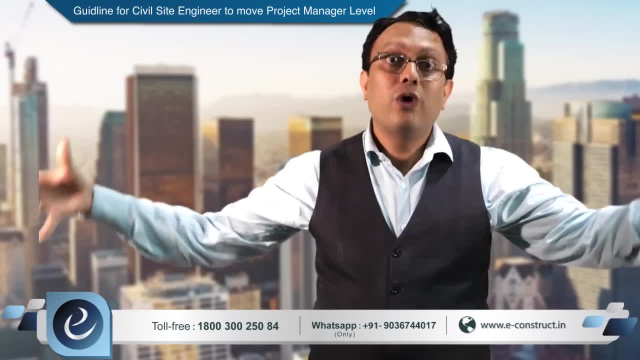 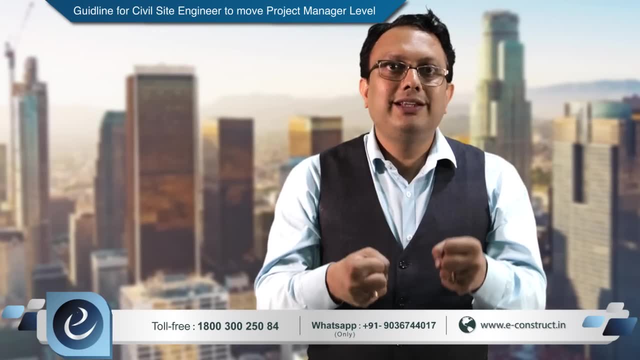 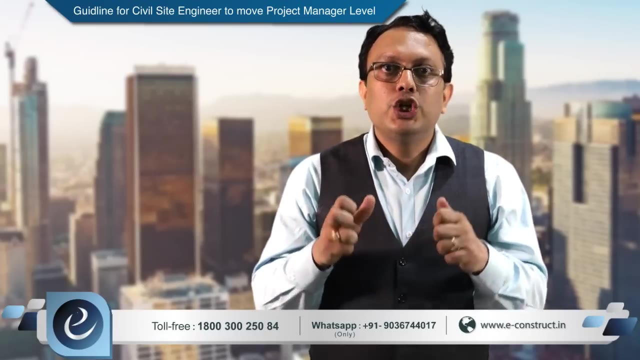 many people has to work together, not against together. work together, together as a team, as one single team. why sport? sport will teach you so many things. football, cricket team: it's not the one person's winning, it's team winning. all right, so make certain activities which will inspire the teams to work together. 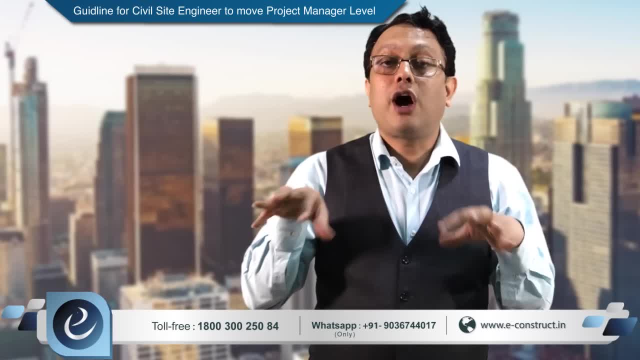 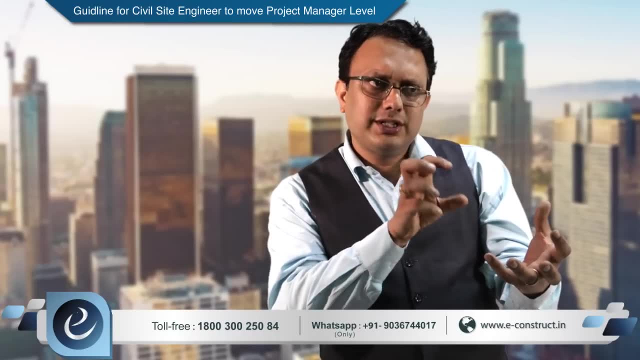 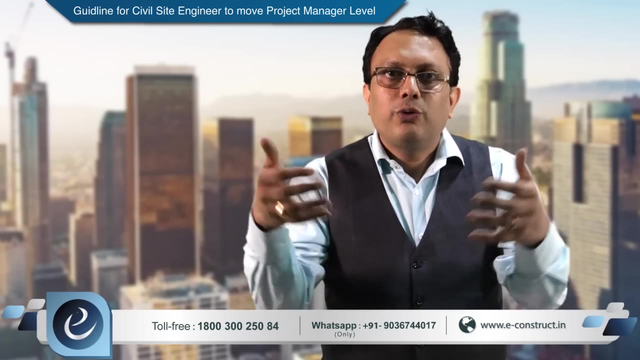 not against together. all right, so how to do the team building? have certain chit-chats, have certain problems. talk to them about the solutions which the problems they are trying to state. try to find out the solutions. when there are certain findings or certain things happens, actually try to make sure that. 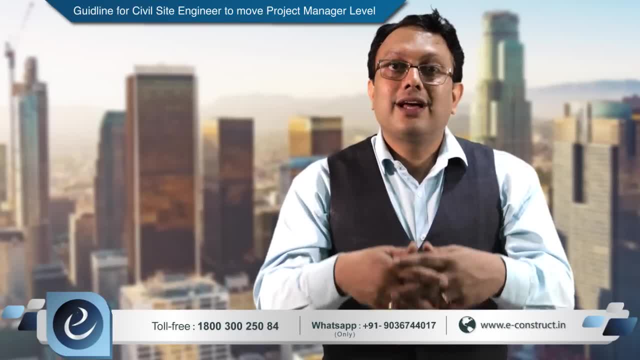 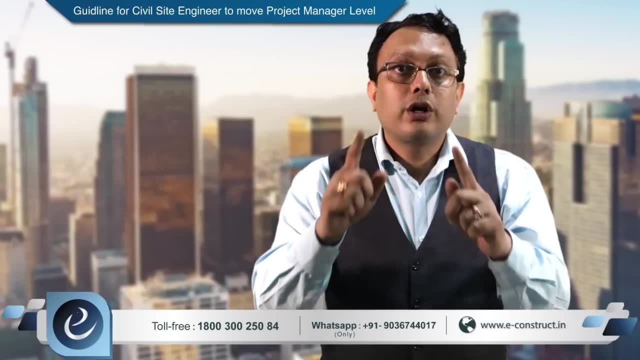 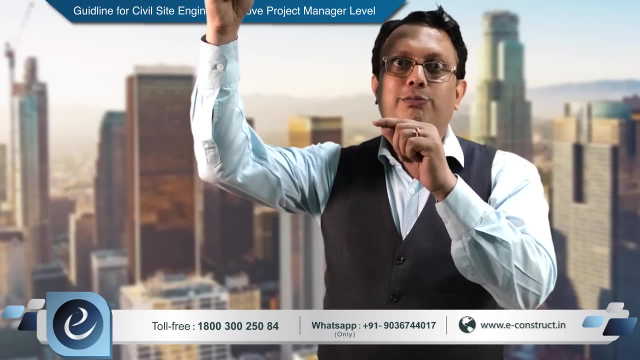 you are working together. if you are thinking that these are hopeless teams, actually try to get rid of it. get the new teams. you are problem solver. you are not problem creator. this game will take you to the next level, from site engineer to the project is all right. the next topic is commitment. you need to be. 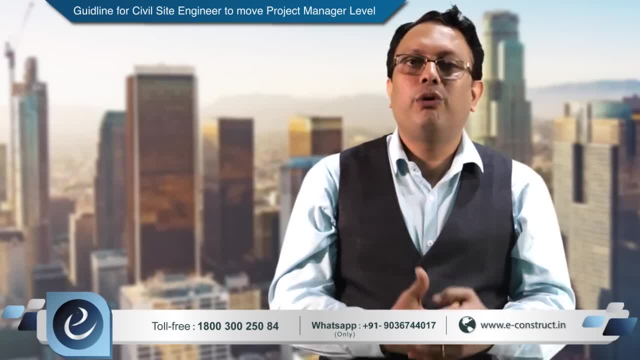 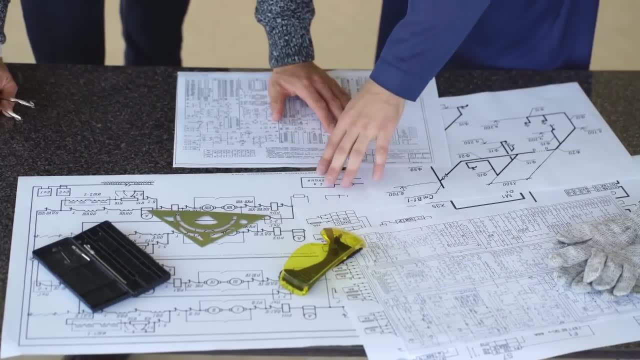 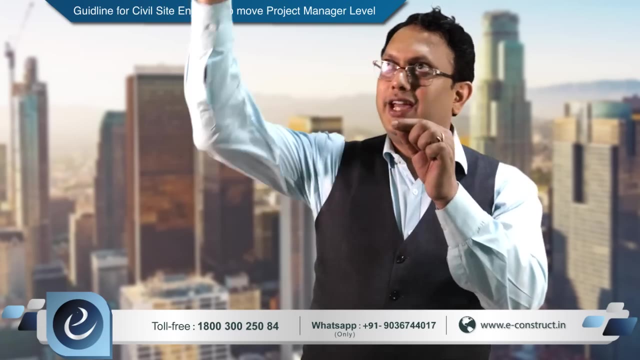 committed person. commitment is very, very important. whenever you're taking any project, be committed to finish it. be committed to do it at in no matter what is the cost to it. when you see that I want go from here to here, this is the place. now you are working with one project and dozens of projects will come. 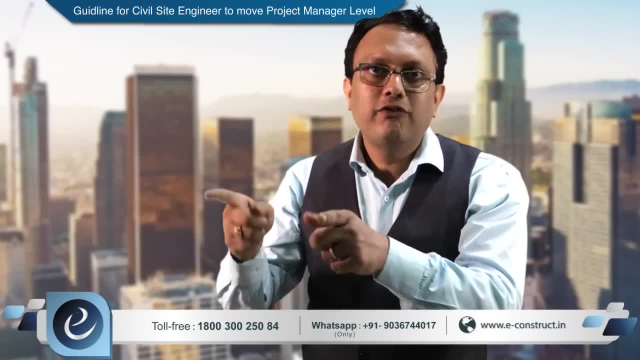 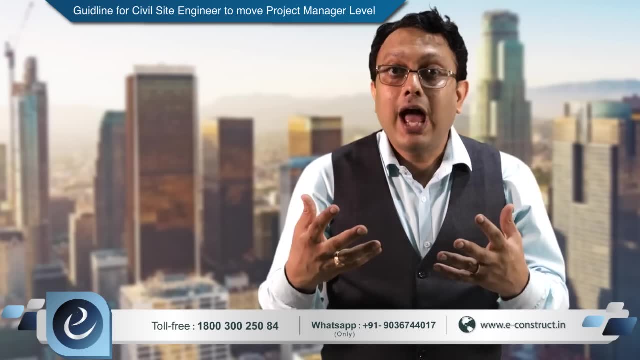 once you complete that, within the budget, within the time frame, within the particular particular limited amount of resource, 10 more projects will come to you. how it will happen? ultimately it will happen. god will give you that. i'll tell you that kind of power will be there. 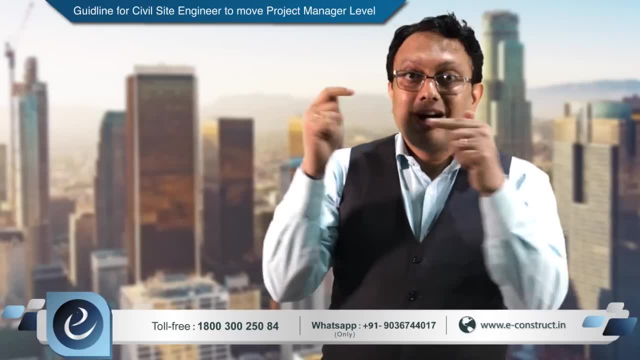 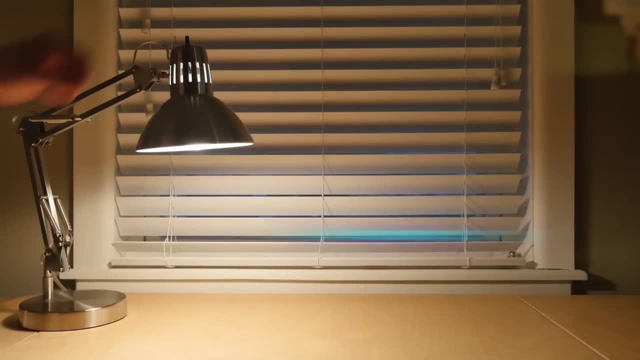 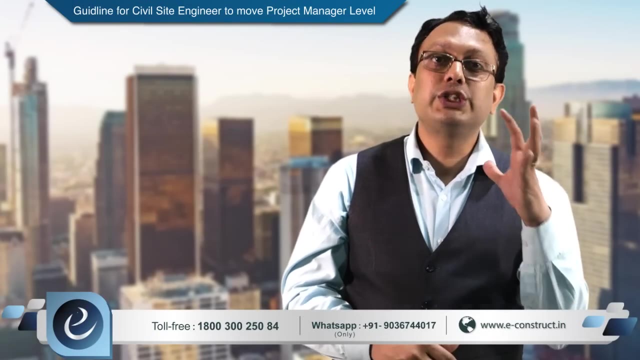 within okay. so always remember, proper commitment to your work is very, very important. all right now. the next point is diplomacy. now, diplomacy is also one of the very, very important thing now. let's say, for example, if your boss is very angry, it's better to give some time to reduce that anger. 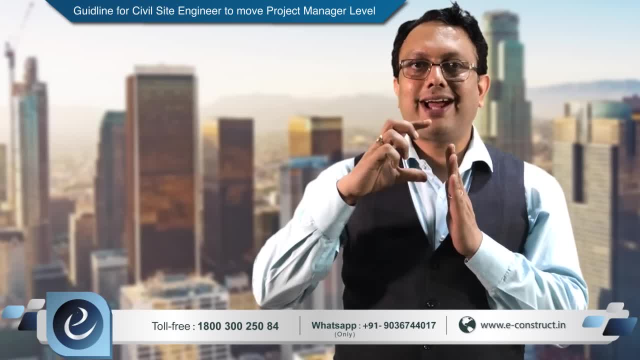 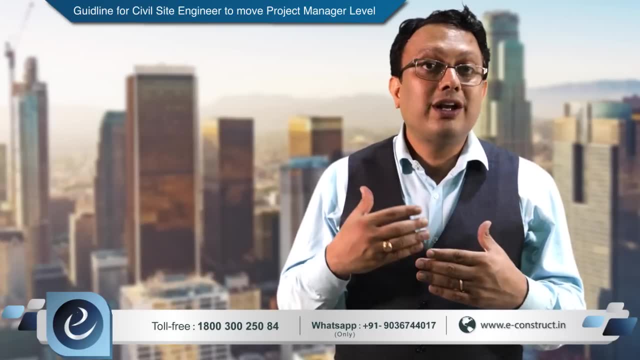 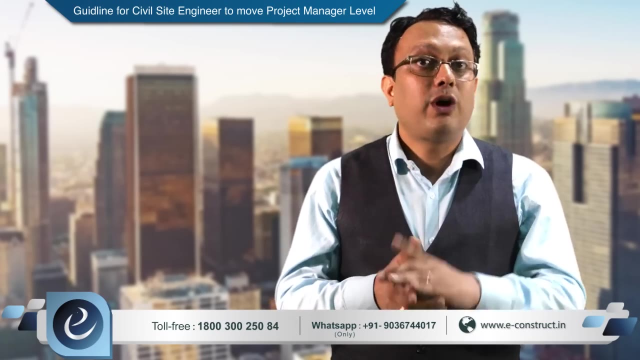 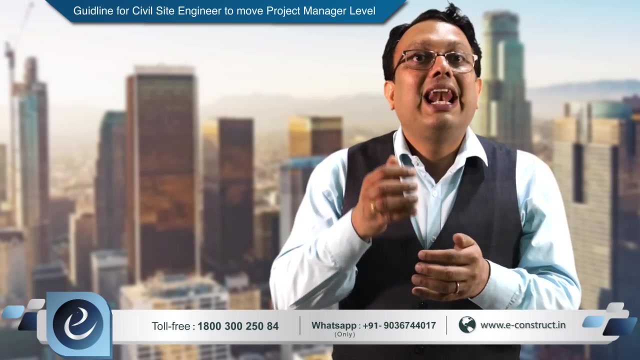 instead of bringing certain problems and make that anger as a big, big, big, big monster. all right. so diplomacy means not a politics. diplomacy is solving the problem with the polite with less amount of friction. always remember: diplomacy is not a politics. diplomacy is solving the problem with less amount of friction. friction means issues with the people, issues with the 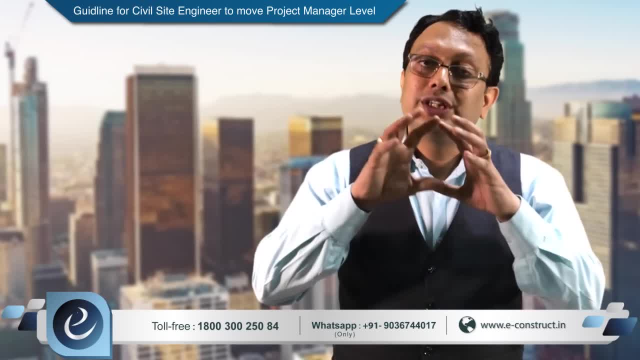 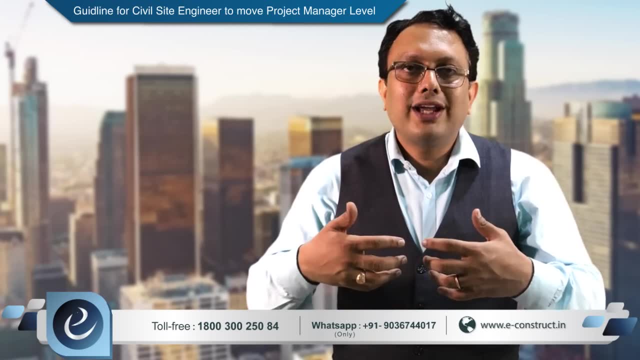 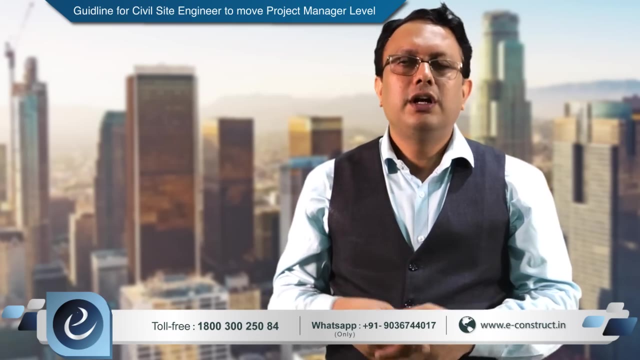 technique issues with the process all right. so these are the areas that you really need to work. actually, how to learn this kind of technique diplomacy requires to be felt within that how to solve this. if you are having the right attitude to solve the problem automatically it will take a. 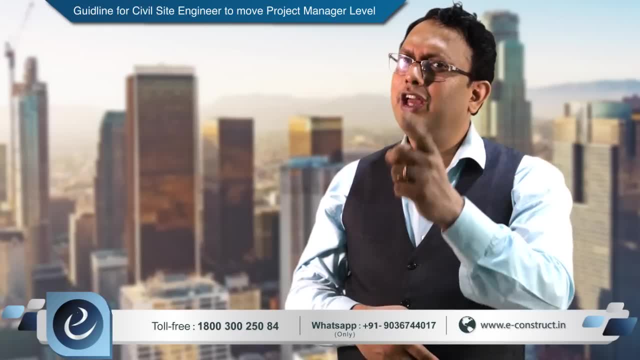 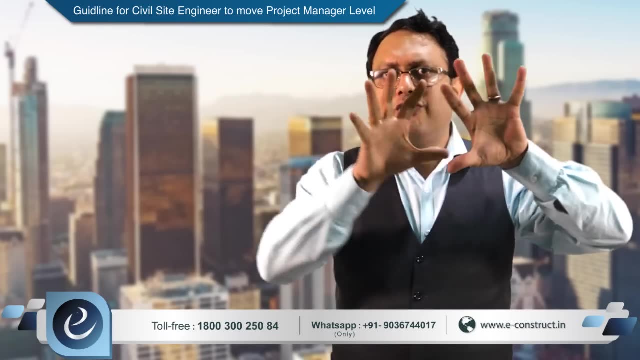 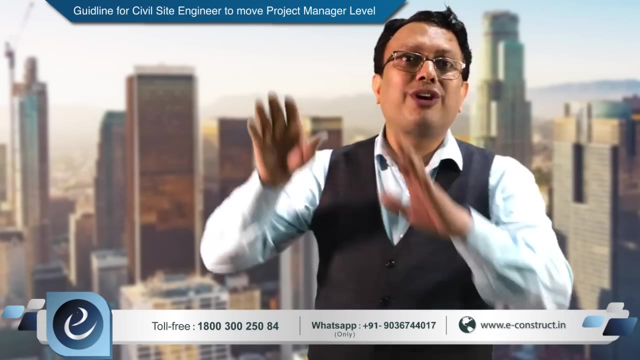 birth within you, but, believe me, this is very, very important quality which takes you from a site engineer to the project manager. now, coming to the different branch, now, these are the behaviorals required, behavioral skills that are required. along with that, you really need technical skills. what are the technical skills now? 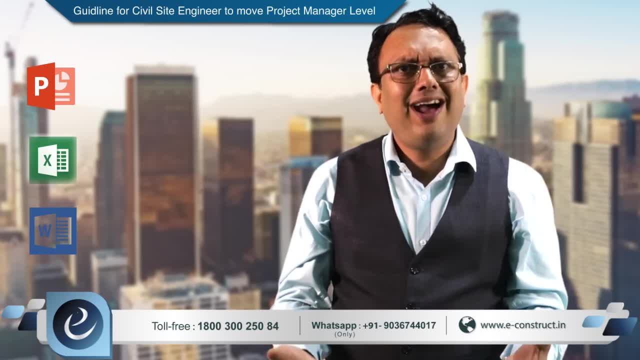 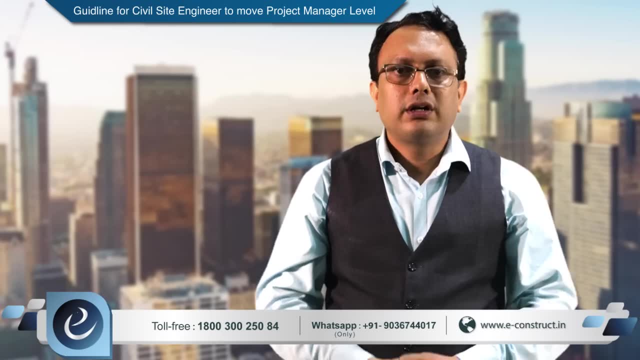 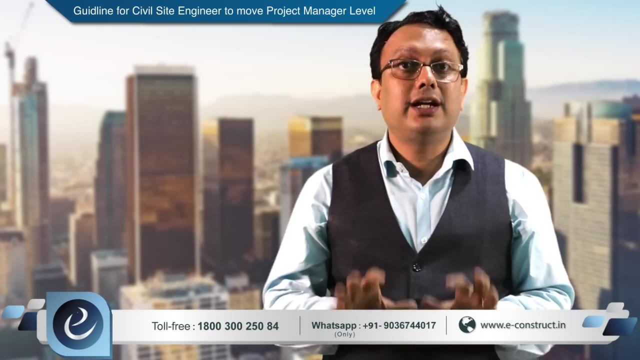 technical skills are like powerpoint, excel. word requires ms office. if you don't know typing, start typing now. type something. write a book on you. type something, your life experiences. start typing. there are so many people: where is a, where is b? that's a problem. start chatting with certain fans. that will also help you. all right, increase your. 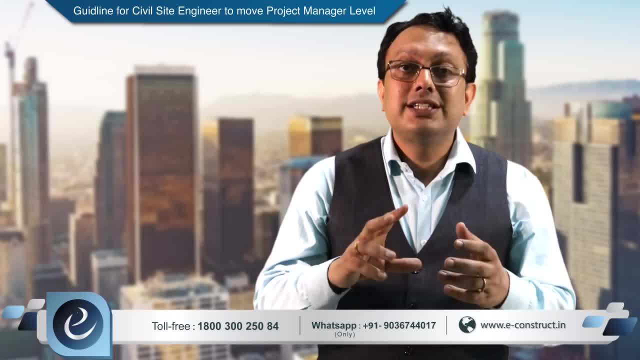 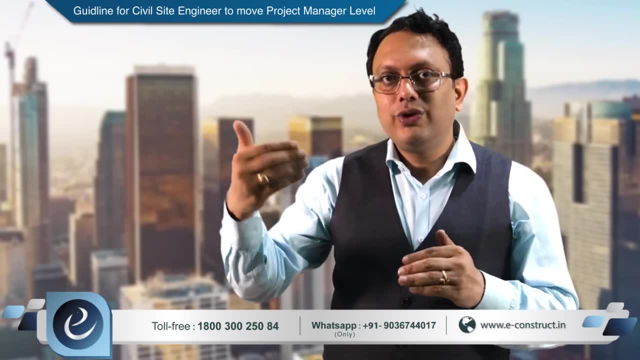 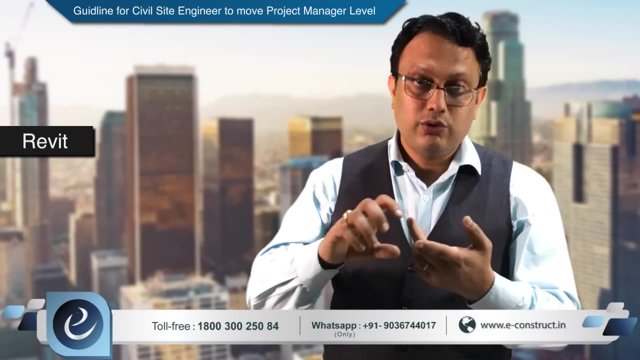 typing speed, first thing. second thing is now. this is about microsoft office. you don't need to go anywhere, you can learn by yourself, right? but certain other levels where you need expertise, that thing actually need to learn. you're required to learn bim tools like revit. you're required to learn certain information giving tools like crm systems. 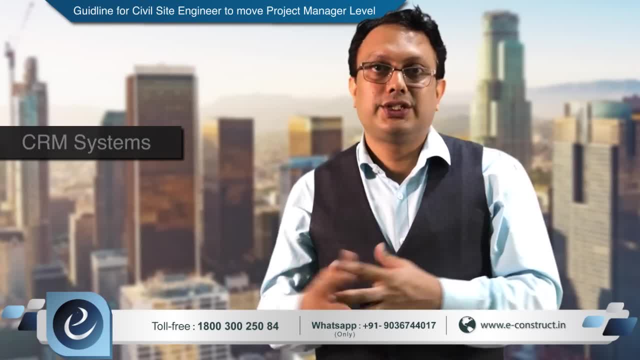 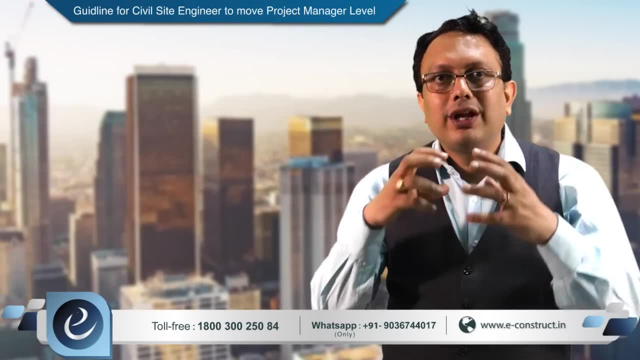 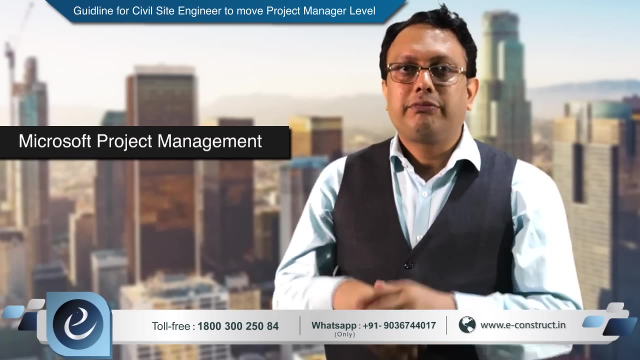 you might be required to learn certain communication systems. now, what all these? actually, whenever you're dealing with certain project management, technical, uh- skill sets, you really need to learn certain softwares. microsoft project management- have you heard about this software? learn it now. so many people actually. they say about primary is better than this. now let me tell you. 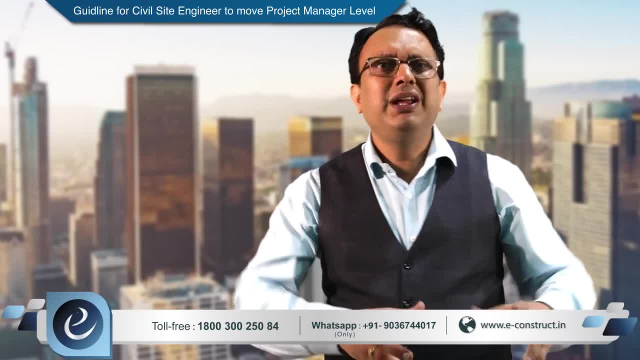 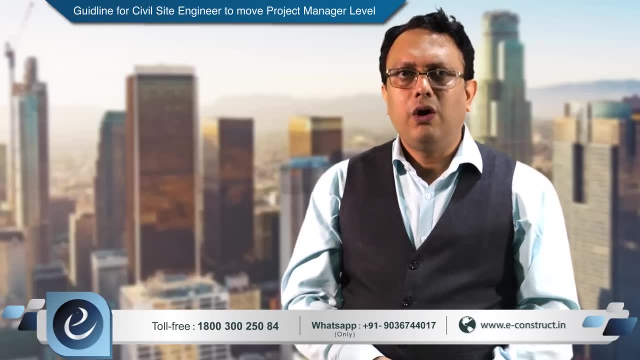 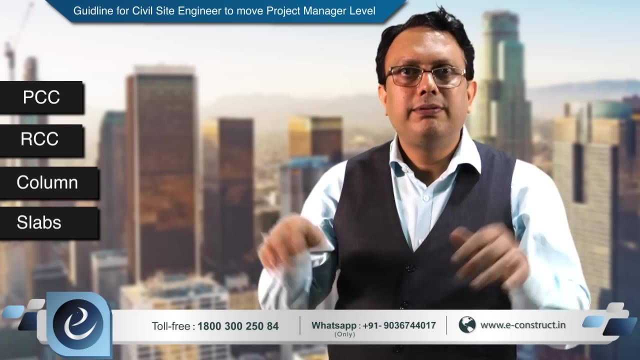 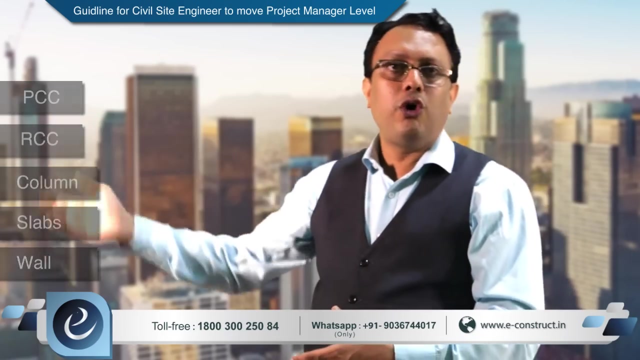 primavera is required if you are having millions of activities. but in civil do we have the millions of activities you tell me? now, let me tell you: you want excavation, pcc, rcc column, then you take slab, you take walls, plastering, painting. why you need, let's say, from office, you need to go to home. 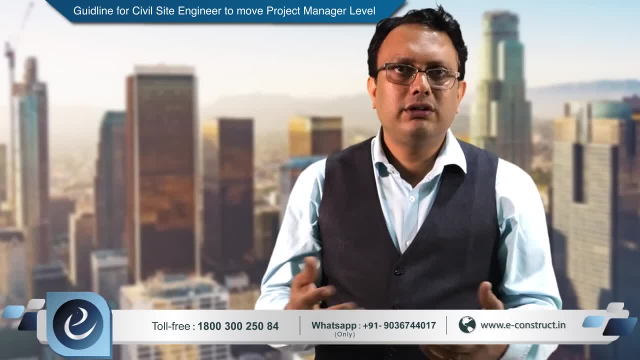 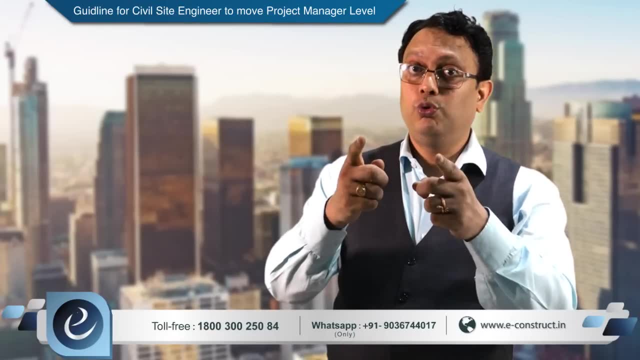 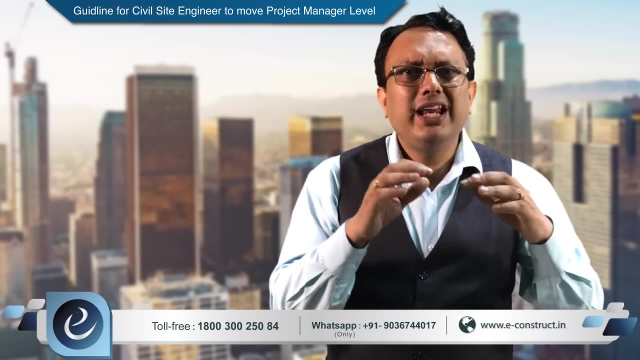 which vehicle you will take. you will take a aircraft, come on, yeah, you will take. sometimes you will walk. if it is just next to your office, all right. so choose the tool, right tool at the right time. microsoft project is comparatively simple tool, very, very subtle, which is compared to the. i mean, like you can compare that with. 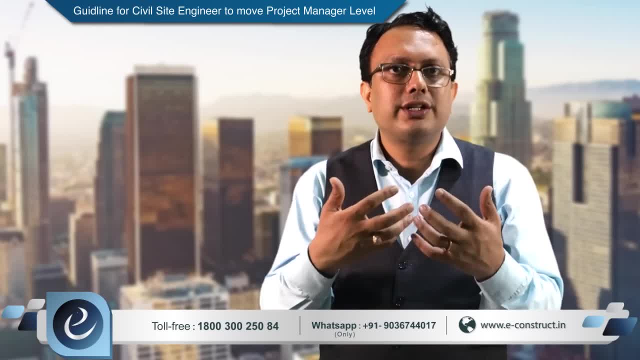 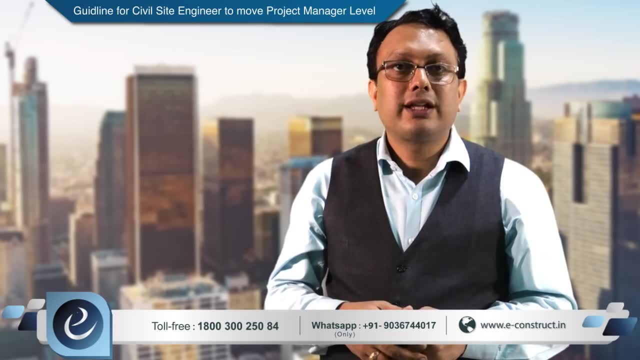 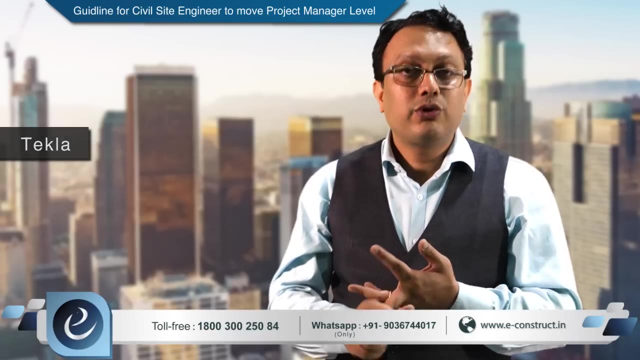 microsoft excel. it is helpful for you to understand certain basic principles of planning scheduling: how to do that, how to learn it all right. few other tools are there like revit is. if you want to do the structural industrial projects. you need to learn tecla if you want. 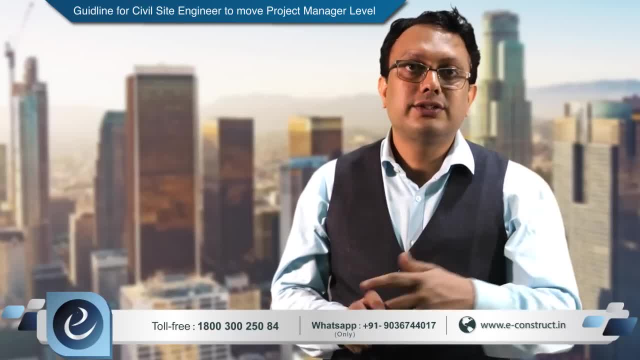 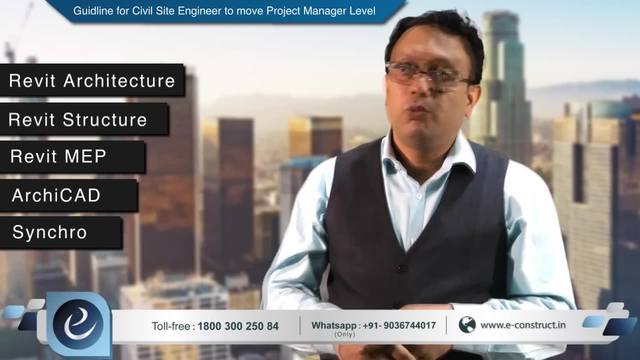 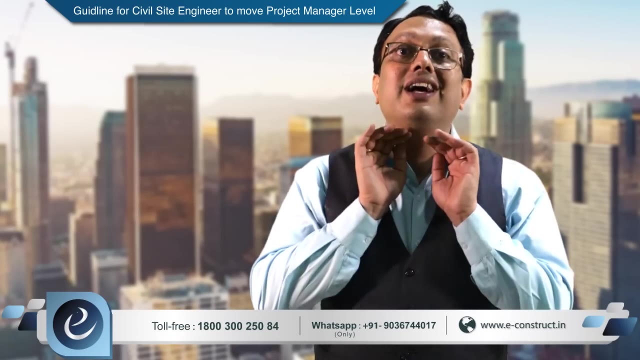 to learn, let's say, the concrete projects. actually, you can learn this. revit architecture, revit structure every time there is archicad. there are various other tools, like synchro- one of the other tool is there, like navisworks. various these tools are there, which will give you a valuable information. 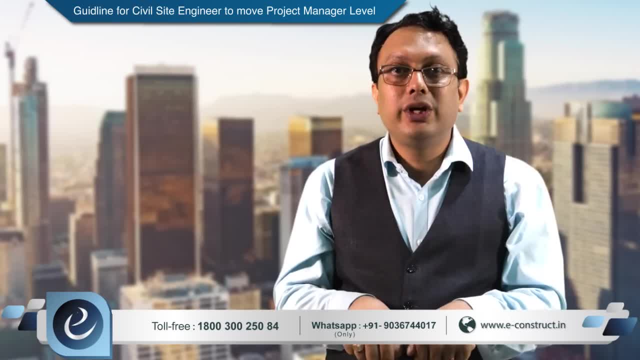 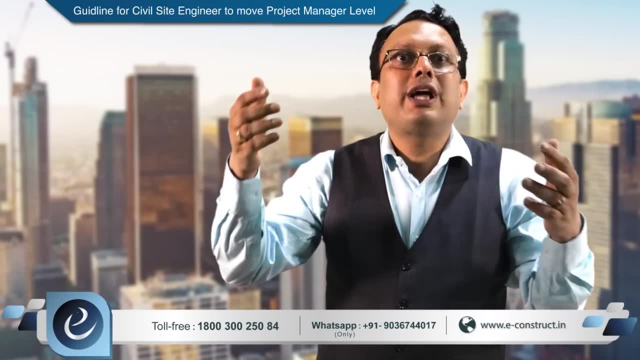 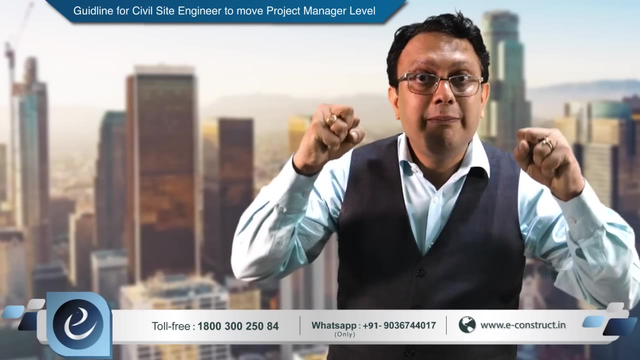 now let me tell you: in today's world, in this century, information is the king. if you really want to become project manager, if you don't have a data, you are not a king. i'm not asking. the king means really the king. i am saying that you cannot be managing it properly, are you? 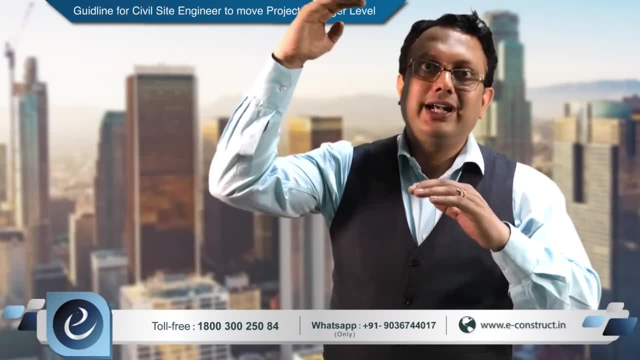 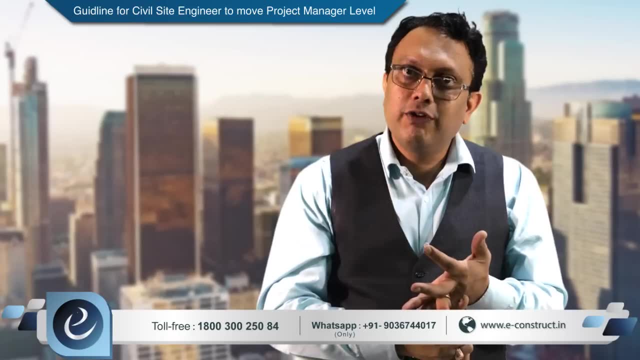 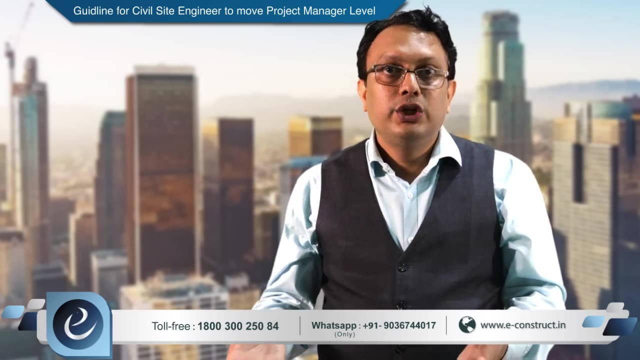 getting what i'm saying. yeah, so whenever you deal with that kind of project as a manager, you are managing all the things. you require funds, you require equipment, you require resources which are related to the materials, which are related to the labors, you require contractors, you require engineers, you require 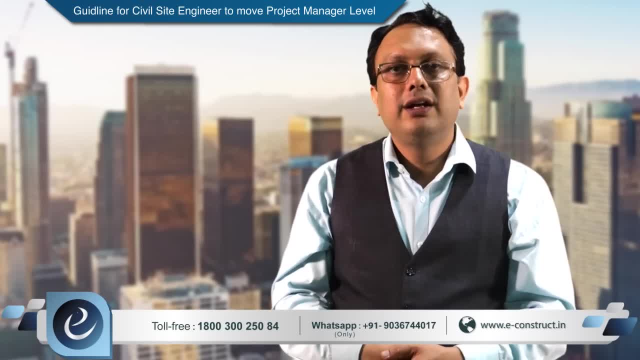 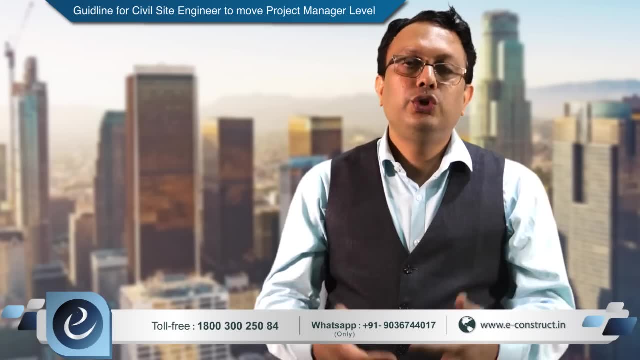 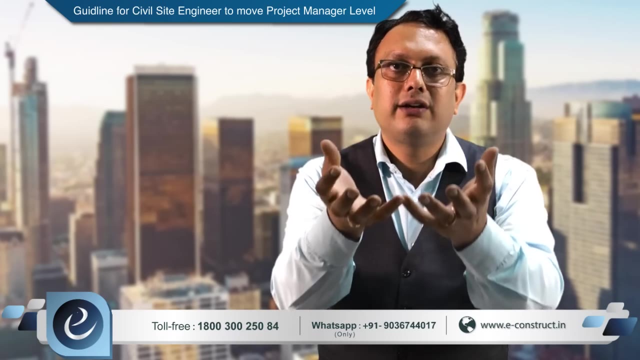 right attitude of the people who are working day to day. you require right staff, you require right accountants, everything. if you really want to work together, you really need a certain type of system which, holistically, will help you and will give you the right information, and that